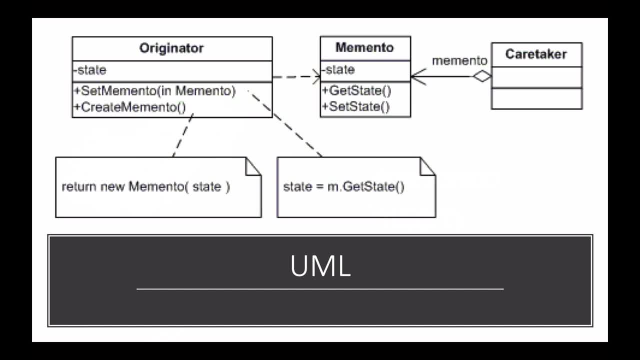 the first entity is the memento itself, and what memento here means is that memory or state you want to save. okay, So memento is the actual state, which we will be persisting. The second entity is called the originator and the originator. 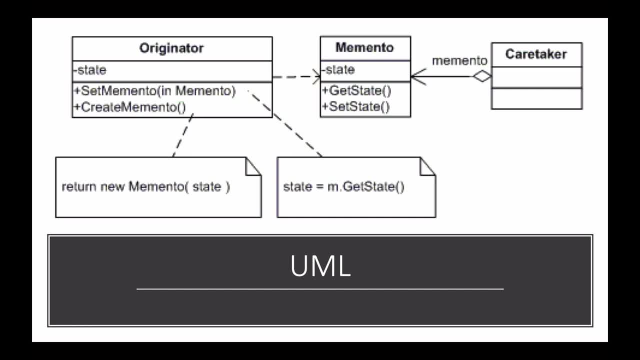 only job is to create and state. the originators is acting like a memento generator or memory generator. what originator will do is it will generate memories, and the third entity in this UML diagram you can see is a caretaker. so what caretaker you can imagine? it's like a picture diary or a photo book, and 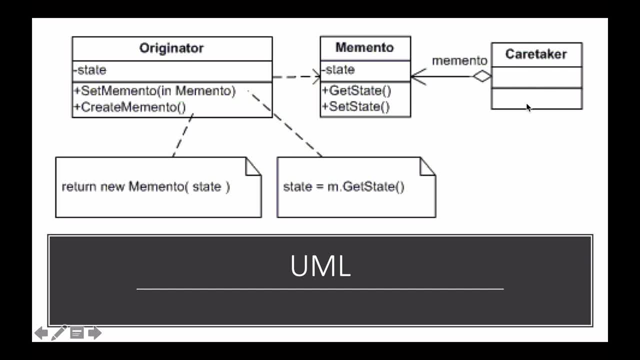 you can save all these memento states inside the caretaker. so caretaker will not have any way to change the memento states. we should not. we will not be providing any way to actually modify the states in the memento via caretaker. the caretakers only responsibility is to have a set of memento memories for an. 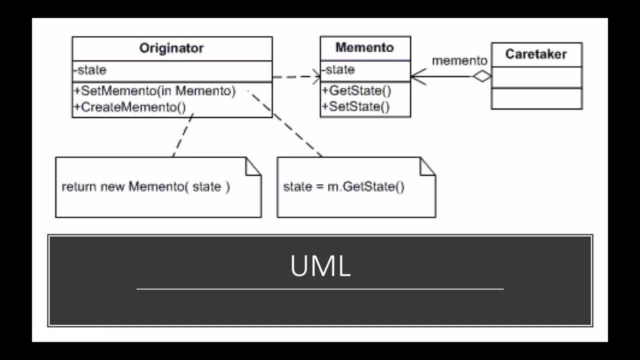 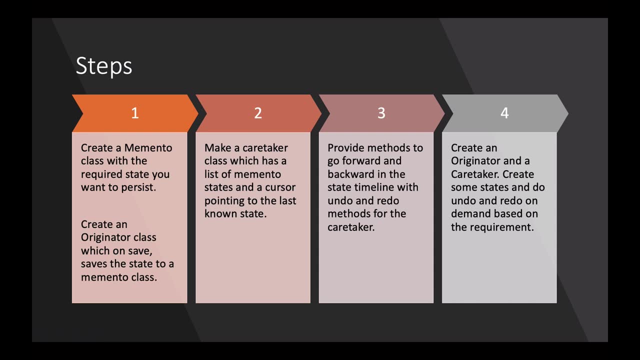 object. we are trying to persist. so this is what the UML diagram means. now let's take a look at a set of steps which will help us to actually implement this pattern. so I have broken down the implementation for memento design pattern in four steps, and here they are. so we will go through each step one by one and make 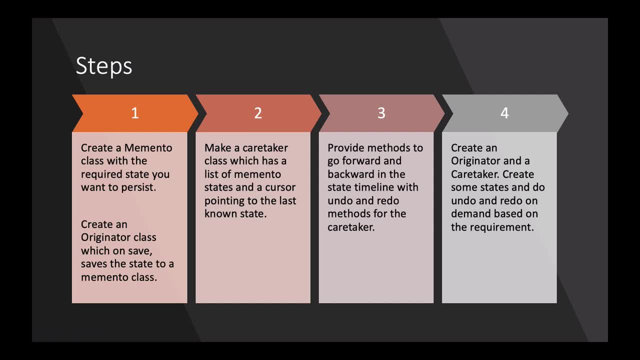 decisions according to the step choices and finally, at the end of step four, we will be having a complete implementation for this memento design pattern. so let's start with the first step. so the first step says: create a memento class with the required state. you want to persist, so 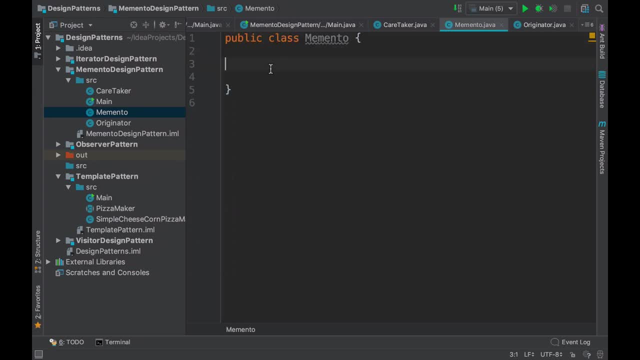 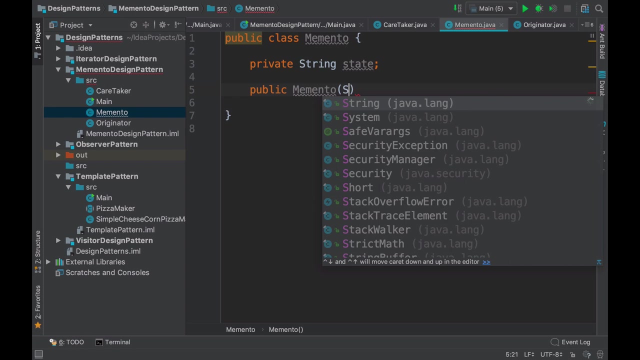 let's go ahead to our IDE and quickly create a memento state, and the state which I am trying to save here is just a simple string. so let me create a string variable called state and provide a constructor for this. so let's take an argument for the state and on initialization, we will set a 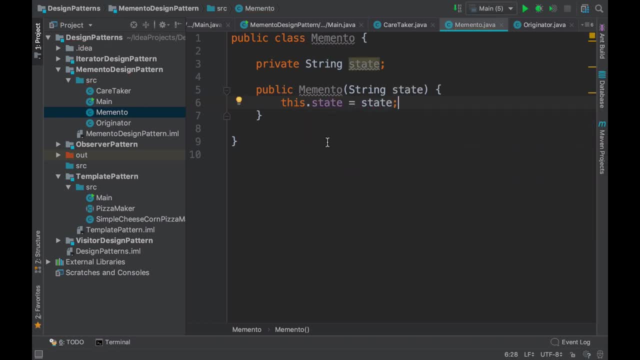 state to the coming state. and this is a very simple class which just holds a string variable which are we calling as a state. so memento is actually a wrapper on this application state. let's also go ahead and provide method to get the state. so say, public string, get state and this will return me the current state. 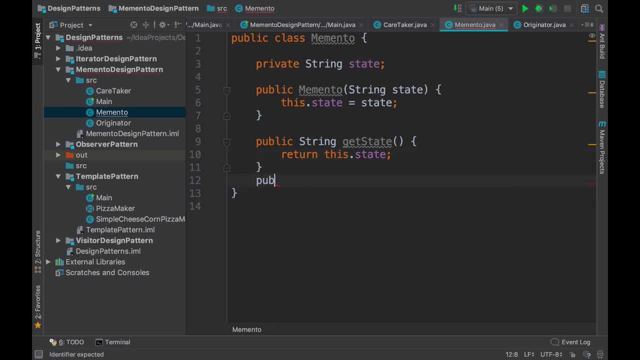 let's add separations as well. so public void set state. this takes a string parameter and say: this dot state is equal to state. so this is it. we have done creating the memento here, and this is the only thing which we need here, since we are only persisting this. 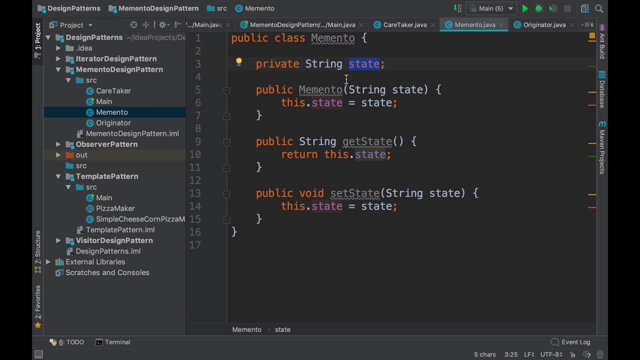 state. we only want to track this changes in the state. we only have one variable here. if your memento, your memento- can be very complex, you can have multiple variables and multiple data types persisted. so for this small example, I am going to stick with this string state, which will have the current state now. 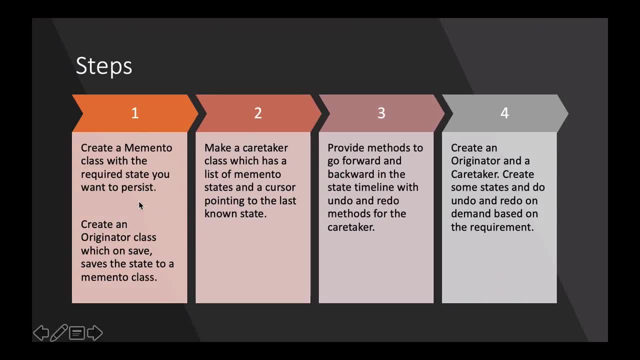 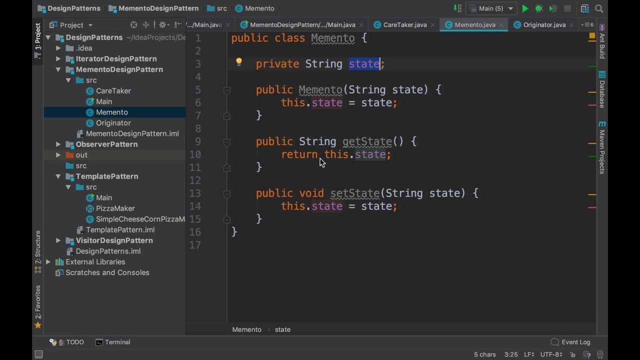 let's go ahead to our steps list. so the first step is finished now. now, in the second part of this first step, we have to create an originator class which, on save save, the state to a memento class. let's quickly go ahead to our originator class. this is our originator class, and 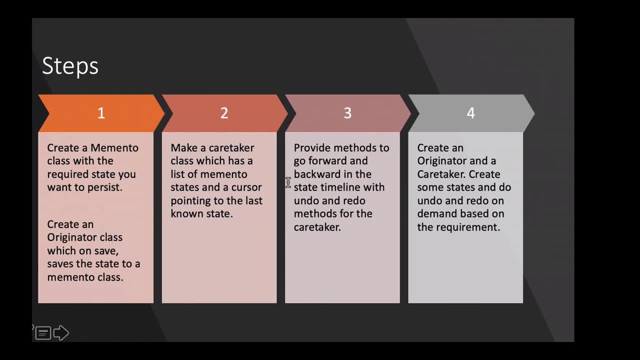 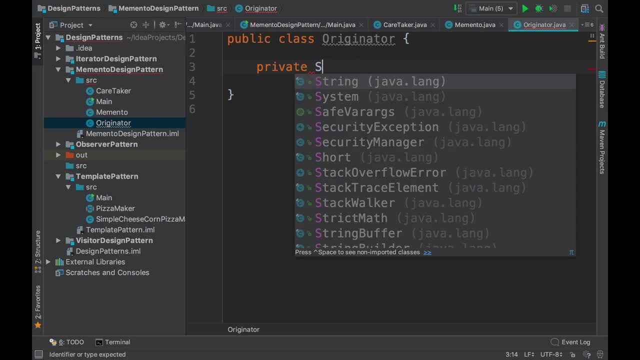 here we are gonna write the code for the originator which, on save, save the state to a memento class. let's quickly go ahead and write it. so for this originator, what I will do is I'll again have a string variable called article and this: 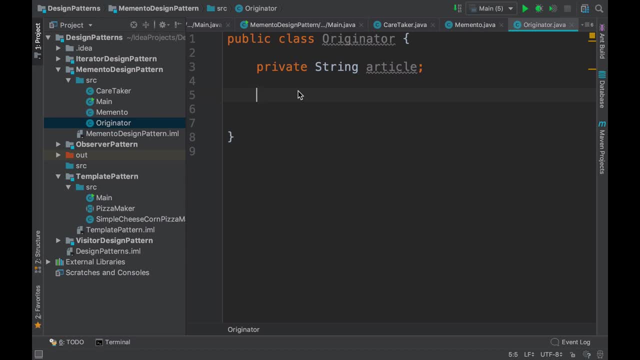 article will be holding the current present article in the memento state. so let's have a default constructor for this, which only initializes it. let's also have a setter for this article, so let's do string article. this dot article equals article, along with the setter, let's go. 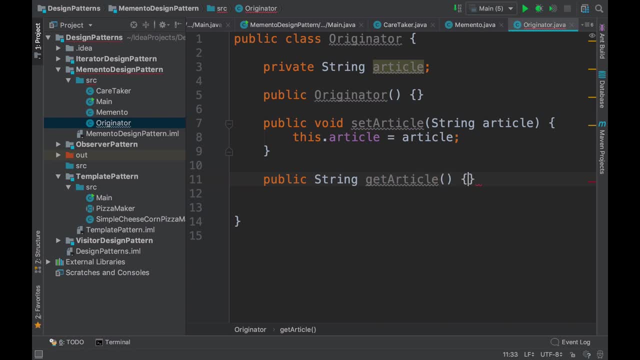 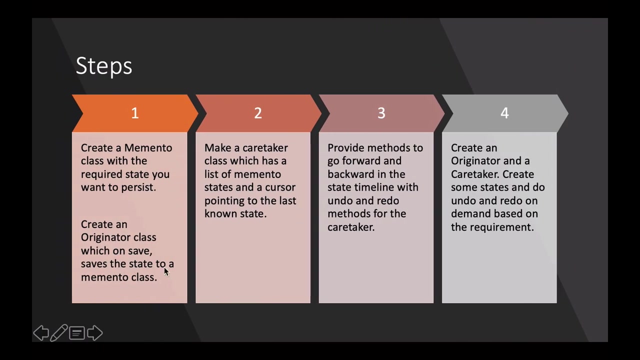 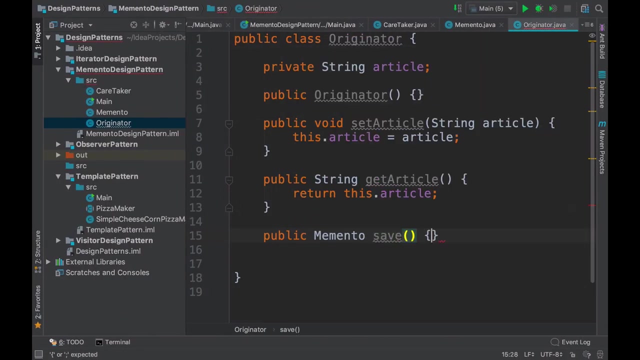 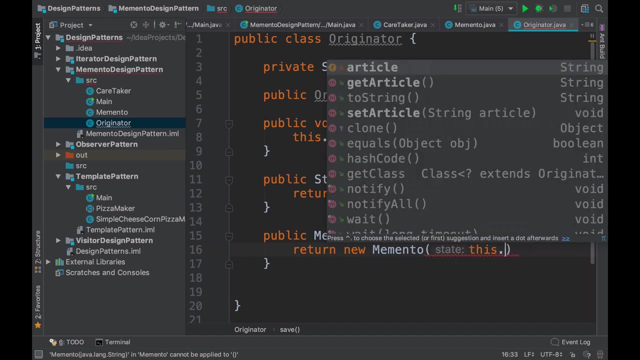 ahead and also create getter, so this getter will simply return me the current article in the originator. now, on save, we need to save the state to a memento class. let's go here and create a save method, and this will return me a new memento which takes the current article. 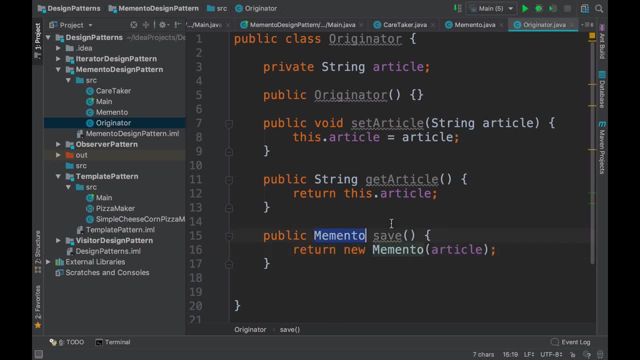 now notice here on save, we are returning a memento object. so once we are implementing the caretaker class and the orchestrator method mean you'll need to- will see how this helps. So we have created a save method which takes the current article from the originator and creates a new memento out of it which you can also imagine as a memory. So 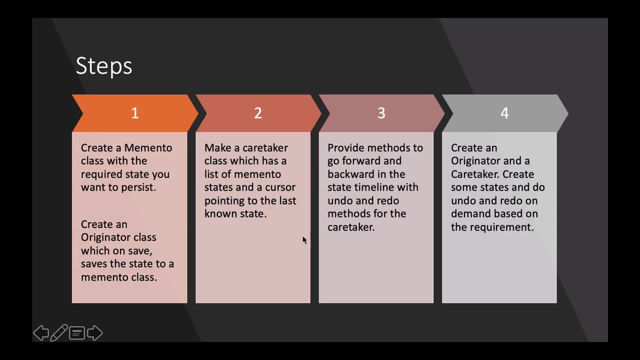 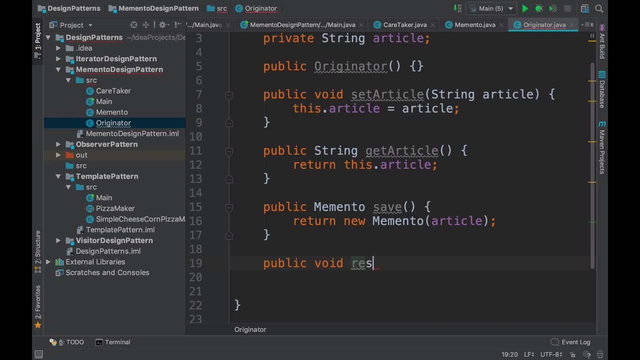 we are creating a new memory with the current article. along with the save method, I'd like to also add a restore method. So what this restore method does is it takes a memento object and resets the current originator state. So what this will do is this will set the current article. 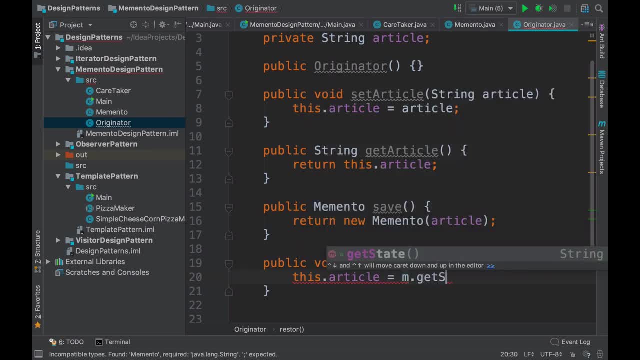 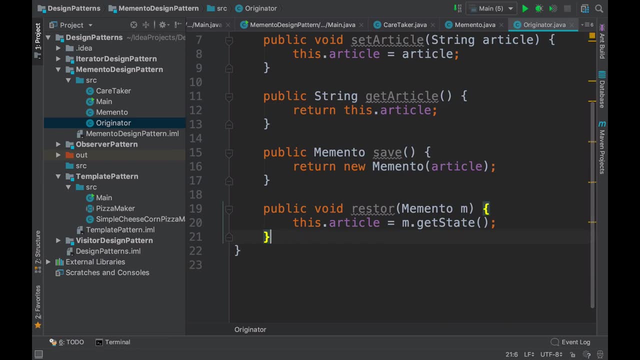 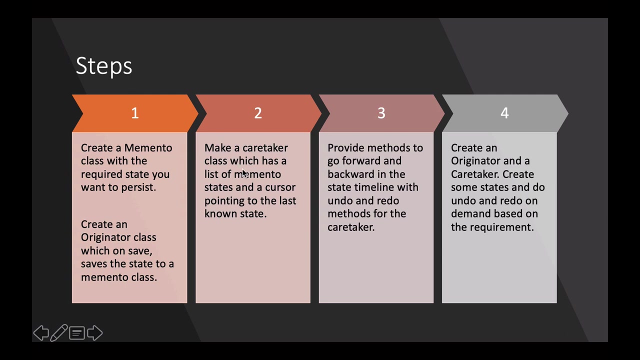 to whatever the state is there in the memento. So now, with this, our originator class is completely coded and now we'll go to step two and implement that. So step two says: make a caretaker class which has a list of memento states at a cursor point. 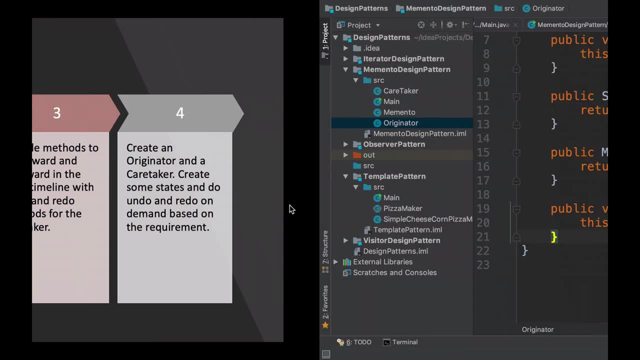 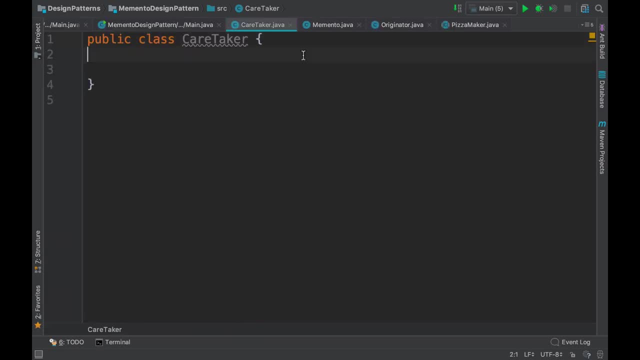 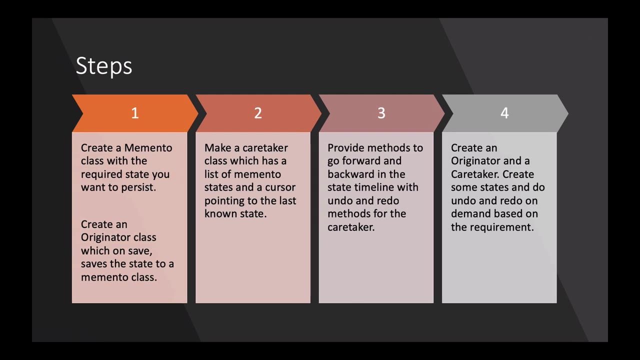 into the last known state. So let's quickly go to our caretaker class, which I have already created, and let's try implementing this. So we will start coding here. So, in the caretaker, what we want is a list of memento states and a cursor point in the last known state. So let's quickly go. 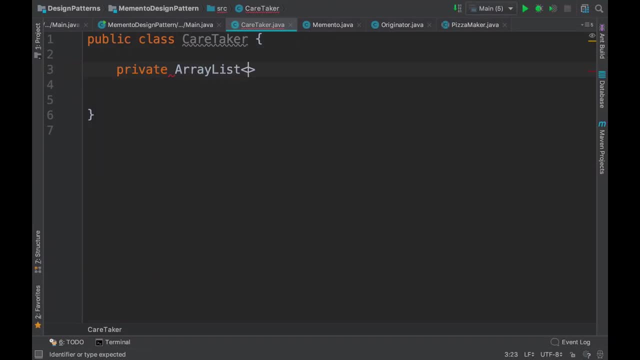 ahead and create an array list which I will be using to store mementos, and let's do an import for this. okay, so now I am calling this state history, so I have an array list which I am calling history and this history. I will be storing all these. 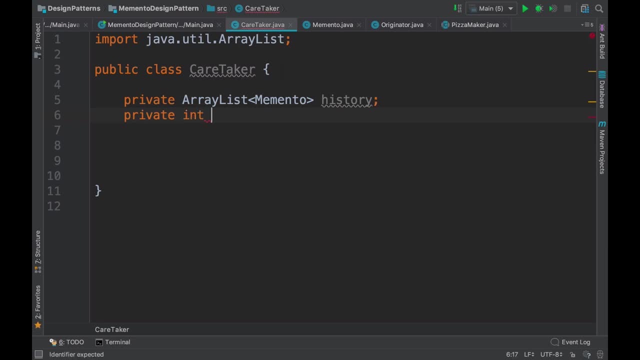 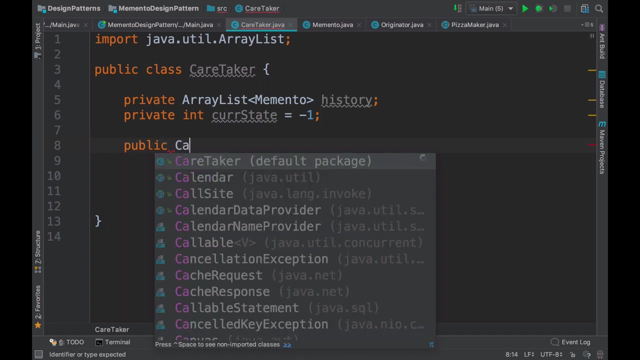 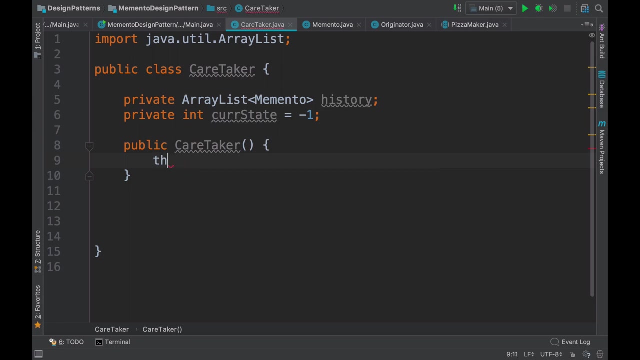 memento states. Now I also want to track the current state in this history object. so because I can go back and forth in this history object, so let's go ahead and provide public constructor and initialize this history object. so in the public constructor we'll be having this: 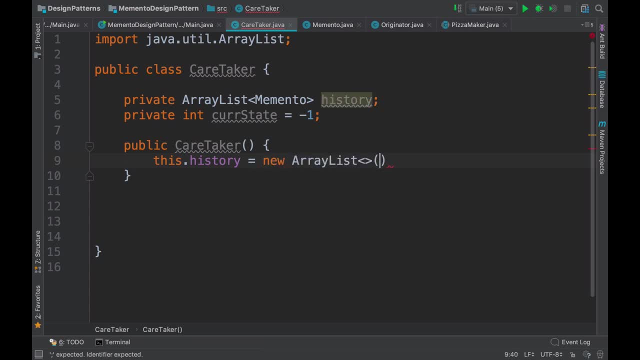 dot history is equal to new array list. yeah, so now we are done with having a constructor for our caretaker. what we'll do now is add method which will add a memento object to this history object. so we will just say public void. add memento which takes a memento, him, and only job of this method is to 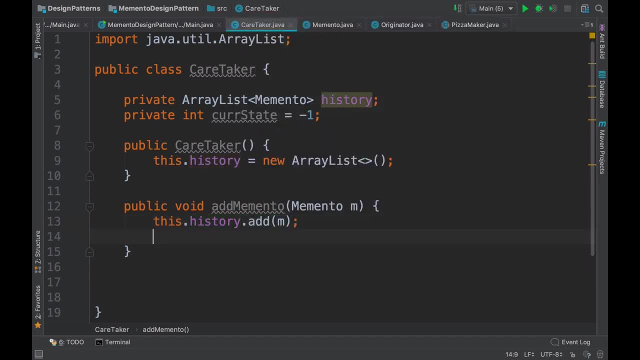 add this memento to the history object. now, since we have added this memento here, our current state is modified now. so this current state is basically storing the index at which our most recent memento is stored. so now this current state will historysize, since we will be inserting the memento at the end of the 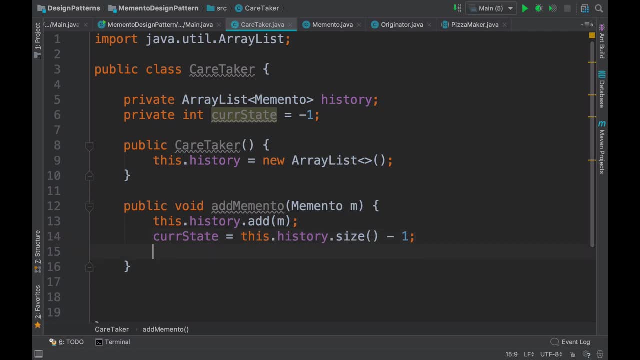 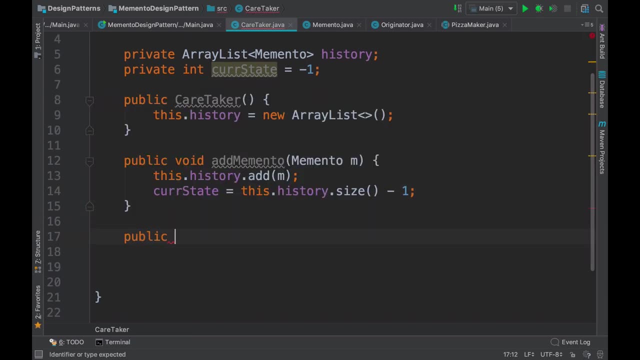 ArrayList. so this is how we can refresh the current state. now let's go ahead and add a method to get the memento, so public memento. since we are getting a memento, get memento, and now we want to return a memento, so we can return. 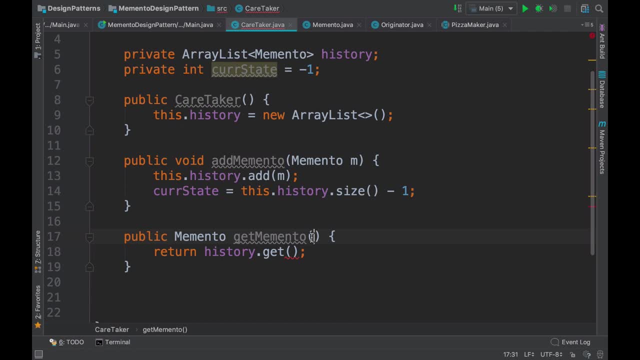 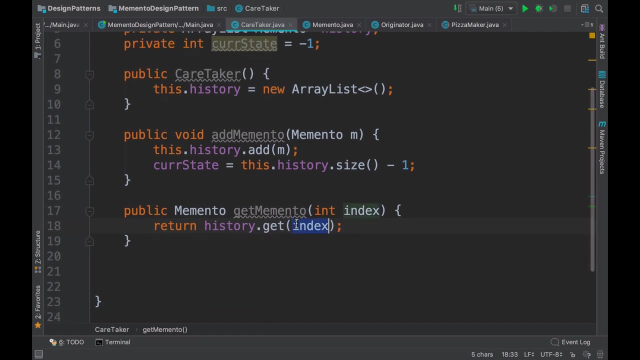 historyget now, since to get a memento we need the index. so we will take an index as a parameter and pass this index to the history ArrayList. so now this will return me the state for which I am providing the index. so now, along with adding and getting memento, let's add the most important piece for 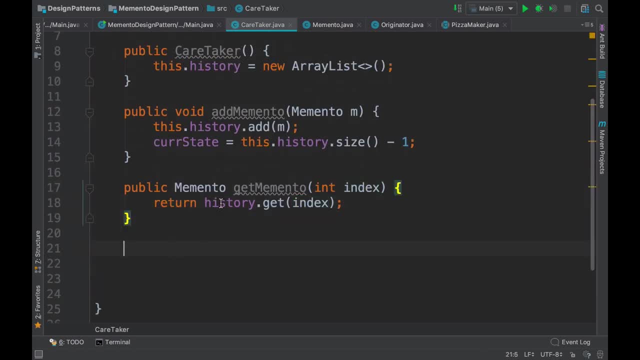 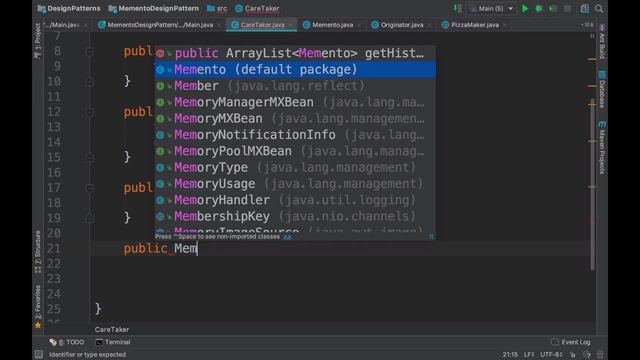 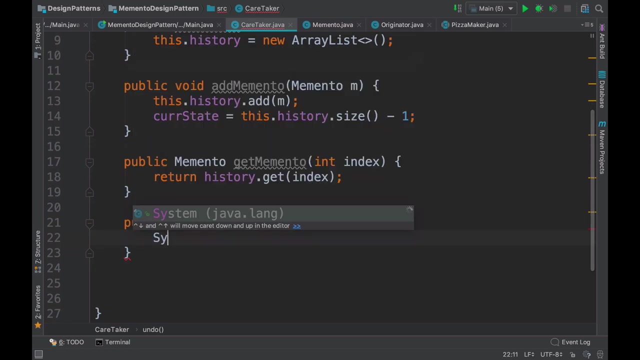 this caretaker which is the undo and the redo. so let's first implement the undo, so public memento, undo. now, inside this undo method, let's print a small logging statement which says undoing state, so we can see that in the console our undo method is being executed. now, if 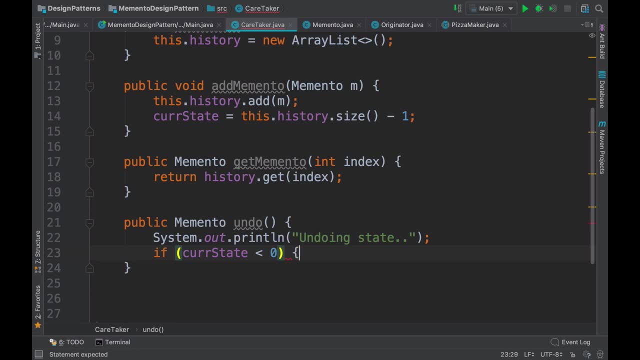 currently, current state is less than zero or it's equal to zero. now, since we are using an ArrayList, we need to keep track of our bounds, so if you go out of bounds, there will be an error. so what we'll say here is: current state is equal to zero, so 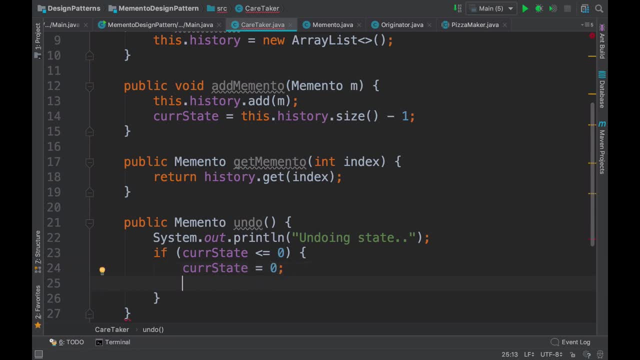 we will not let the state go less than zero and we will return get memento of current state and we will return get memento of current state and we will not let the state go less than six or something like that. as event comes in the data or soon drill it or we will return mean he can and zero cancel. 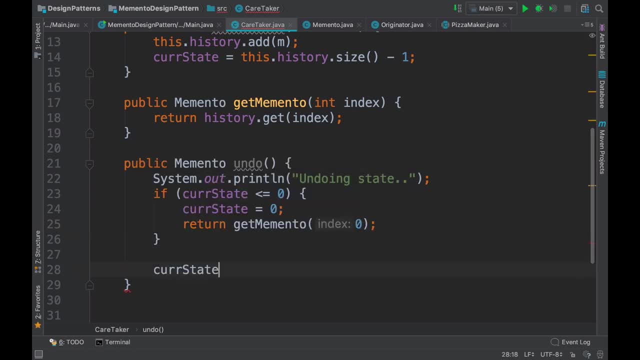 the state or attribute I can say, so that It's two or three, right, two, three, four instead of zero, or zero or 0. you can well, you can. if it's not the case, what we can do is we can reduce the current state and it'll get memento for this. 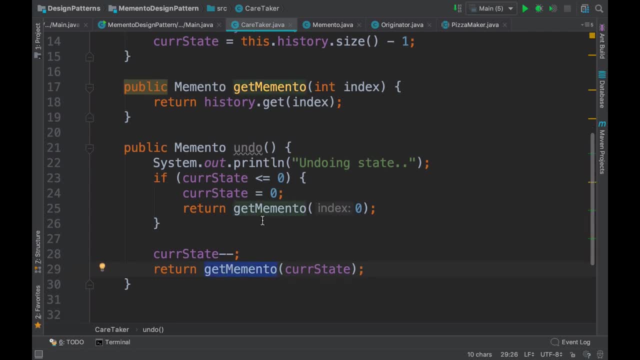 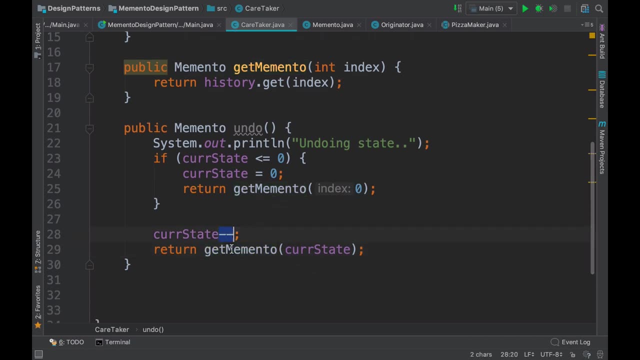 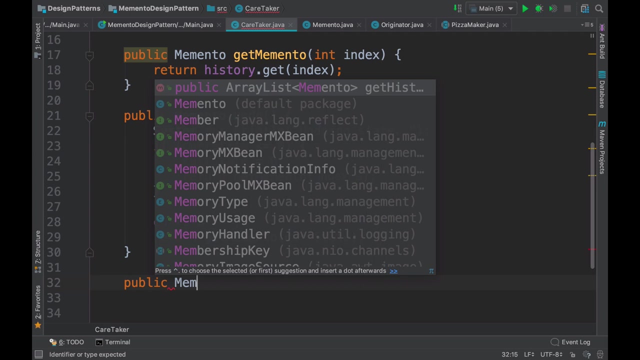 current state. now this memento will return me the last state or the previous estate for the current state, because we are decrementing the current state in this now. similarly, let's go and provide our redo method, so let's go and replace. so redo method will also return a memento and we'll call it a redo. Let's. 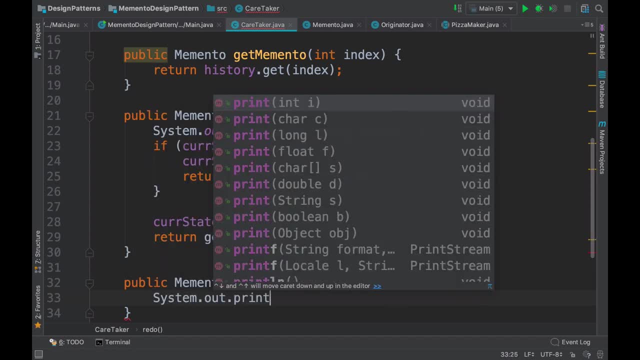 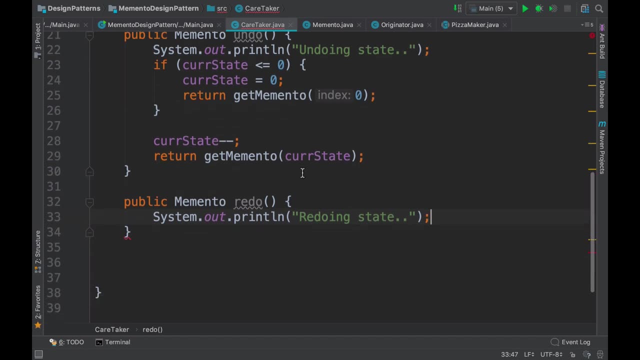 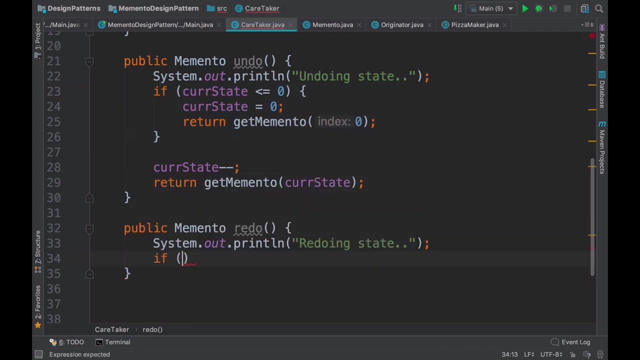 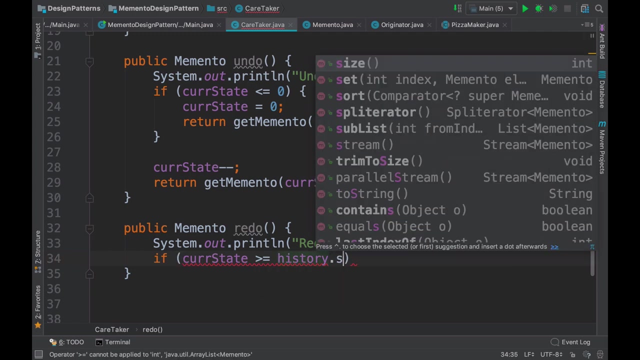 also add a small logging statement here as well, which says redoing state. Now, similarly, as we are looking for the overflow in the undo method, we also have to check for the overflow in the redo method. So let's quickly go ahead and implement that. So we'll say current state if it's greater than historysize. 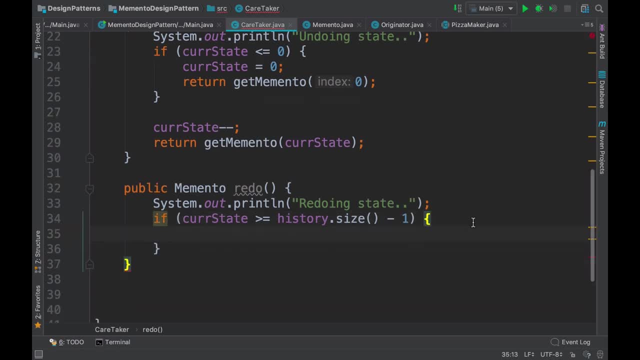 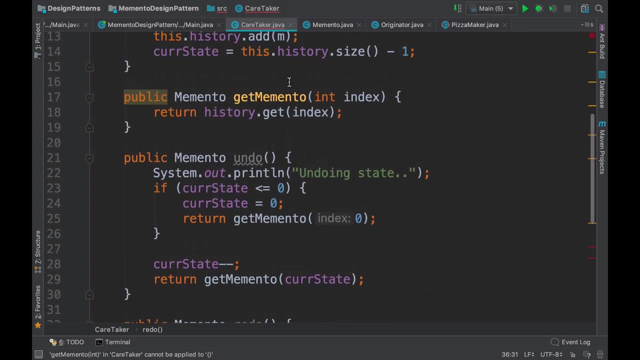 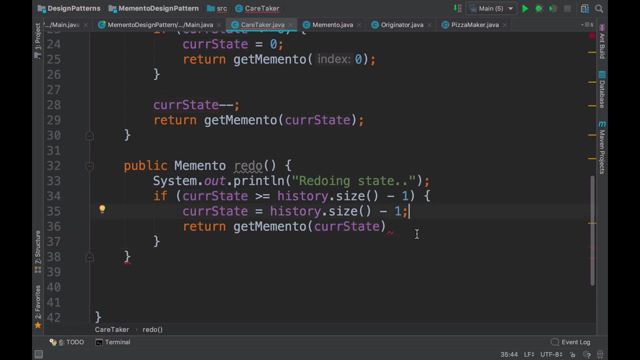 minus one, since we have a zero indexed array. we want to set the current state again to the max value of the history object size, and then we will return the get memento, which is the utility method we created above, and pass the current state. So this is how we'll be handling. 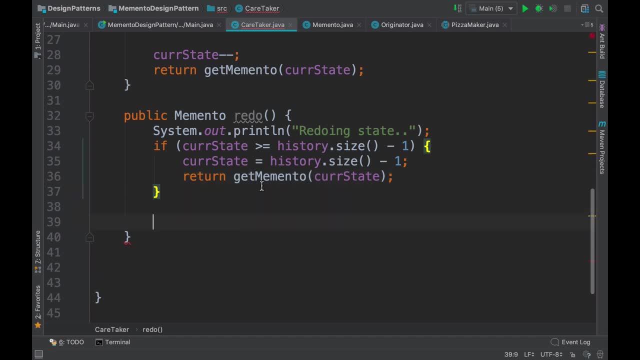 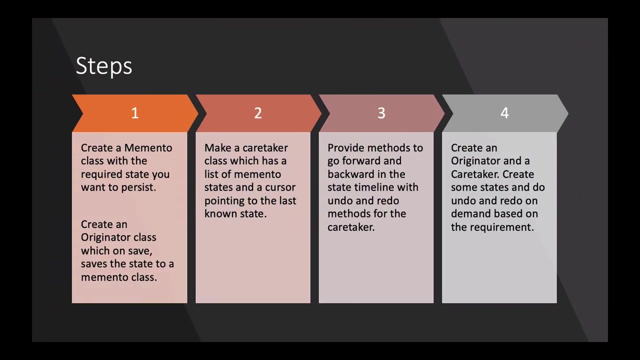 overflow in the case of redo, and if this is not the case, we will simply increment the current state and we can return from the get memento passing the current state. So this is how the redo and undo method looks like. So now we are done with step two, and step three says: provide methods to go for. 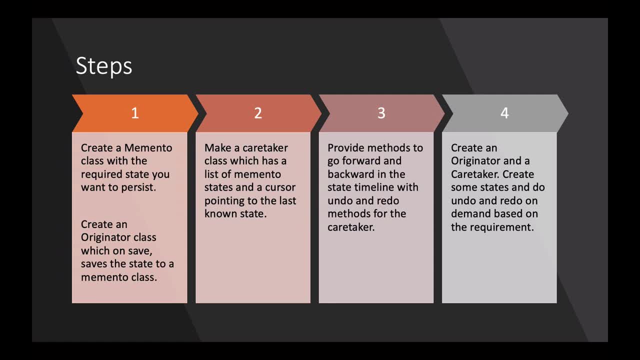 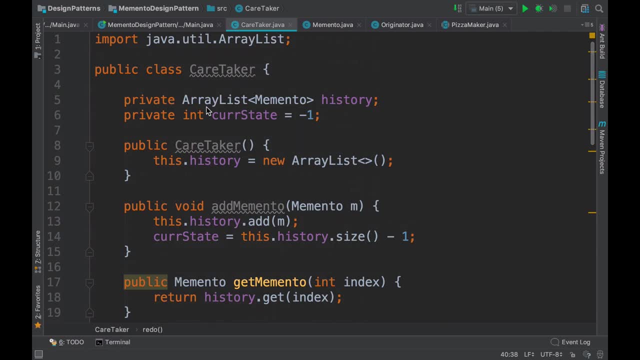 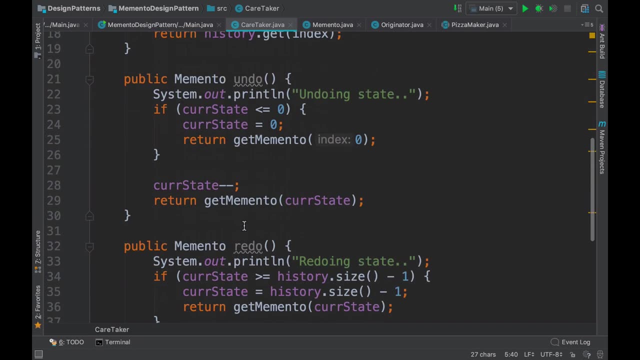 forward and backward in the state timeline with undo and redo methods for the caretaker. So we have also implemented step two and step three. So step two said that we need to create a caretaker class with array list of history objects which will store all the memento states, and step three says we need to provide a 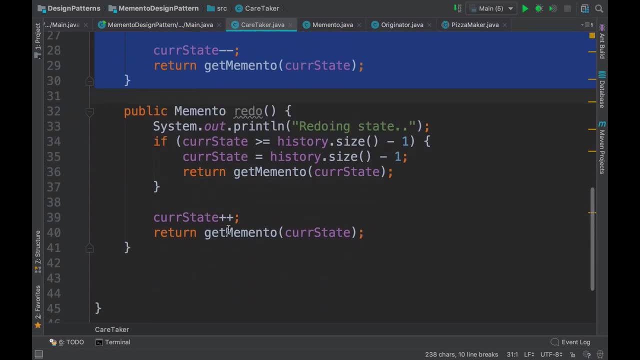 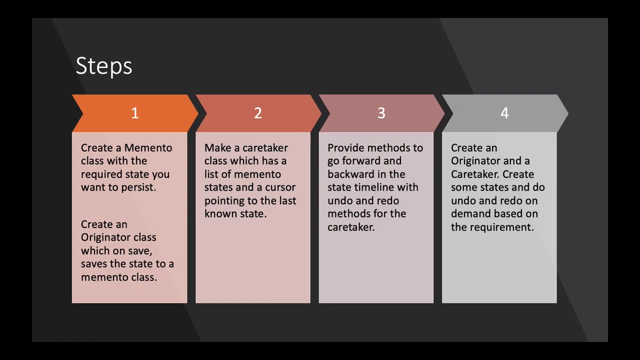 undo and a redo method to actually go forward and backward in the timeline for the memento. Now step four says create an originator and create a caretaker and create some steps and do undo and redo and demand based on the requirements. So now we are completely done with implementing the memento design pattern. 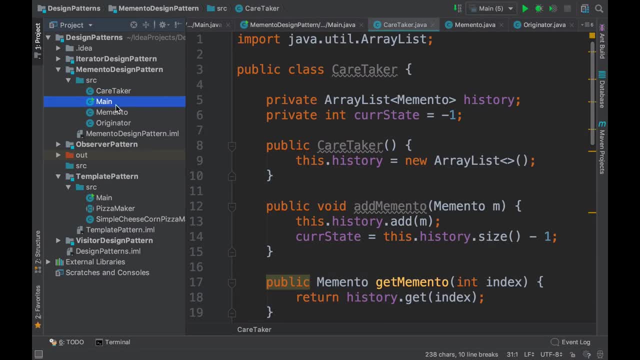 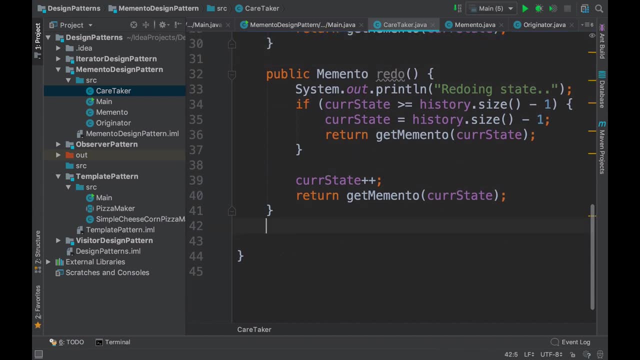 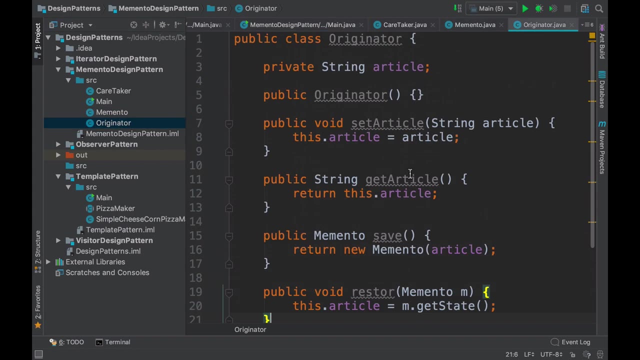 and now it's time to see this in action. So let's go ahead and go to our main method. So let's have a look at all our classes, that they are implemented correctly and all of them looks good, Yeah. so now let's go to our main method and let's start playing with our memento. 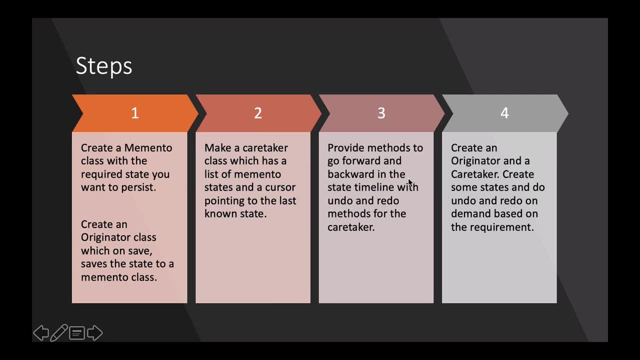 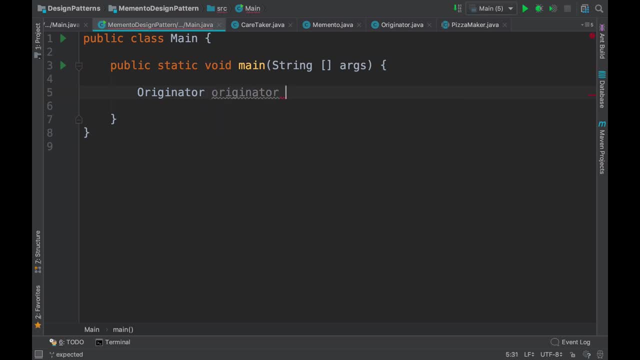 pattern. So, as the fourth step says, we need to create an originator and a caretaker object. So let's quickly go ahead and create a originator- originator or is new originator- and similarly we need to create a caretaker object. So 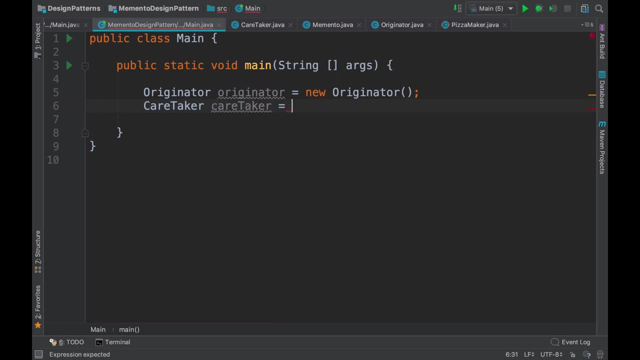 let's create a caretaker. Now we need to instantiate the originators are created. So let's go ahead and set the article to some state. Let's call this state state one. Now, since we have set the article, we also need to save the. 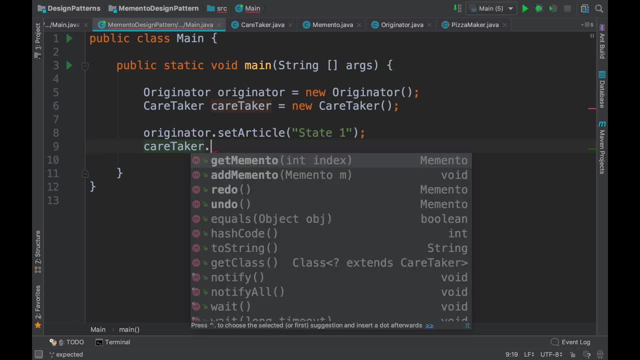 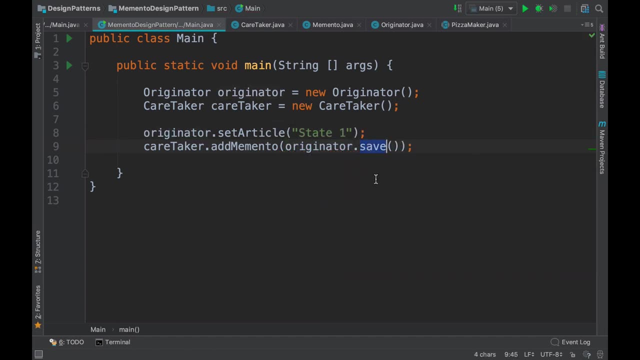 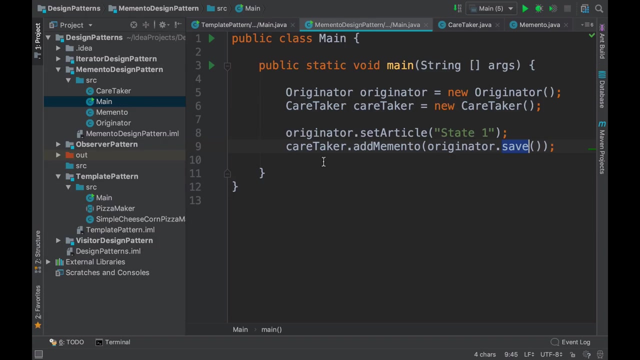 state. So what we will say is: we ask the caretaker to add a memento to its history object and call the originator dot save method. Now, if you remember what this originator dot save method does, it creates a memento From the current article. So now I want to save the current state and I am 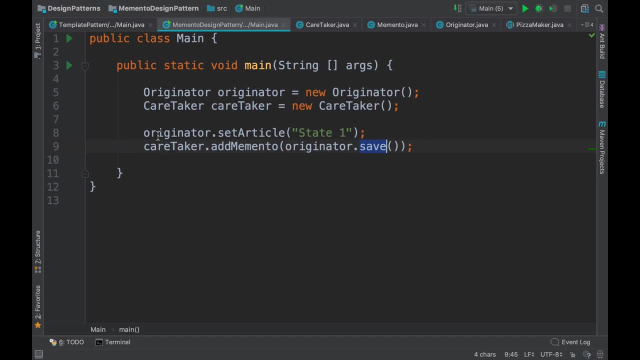 creating a memento out of it. and what I am saying is: to the caretaker object, add this memento written by the originator dot save method. So now I have the current state in the caretaker's history object. Now let's go ahead and implement. 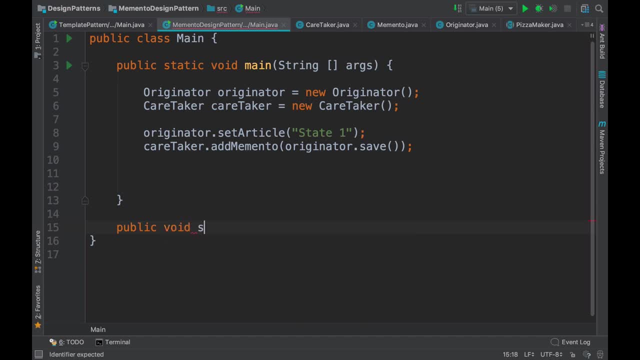 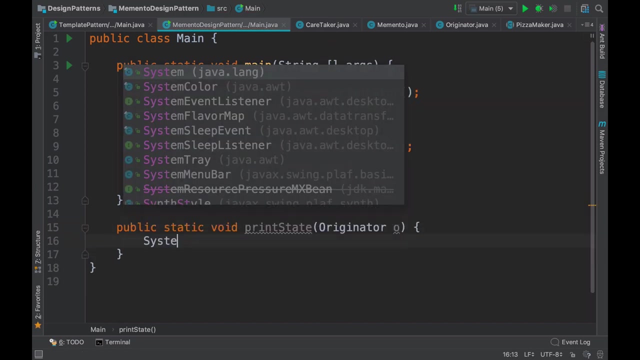 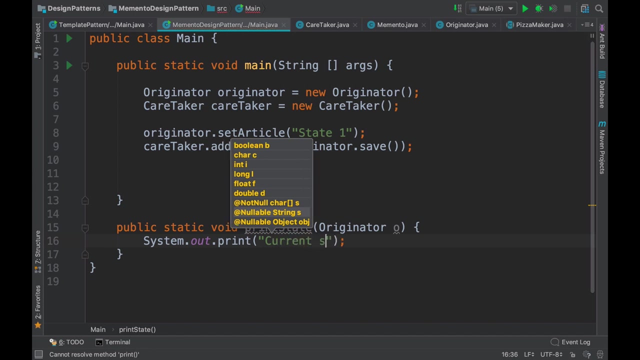 a utility method which will help us to actually show the state for the originator. So we'll say public static void print state, and this takes a originator reference. and what this method only does is it goes ahead and prints to the console the current state and o dot. 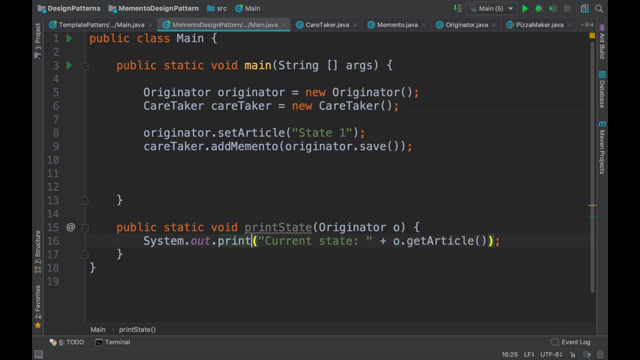 get article. So that's the only job. Let's add a print line here. So the only job of this print state is to show the current state for the originator. So now we have saved this current state for the originator in the caretaker's history object, Let's go ahead and print the state for this. 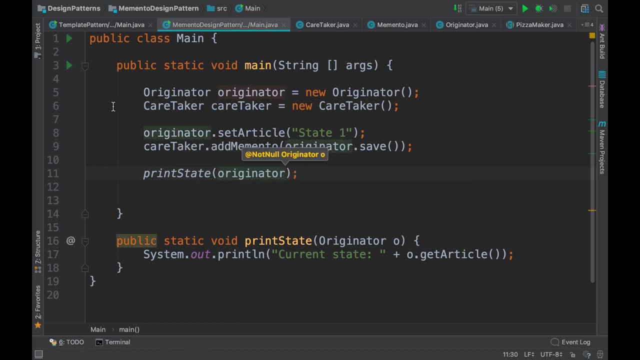 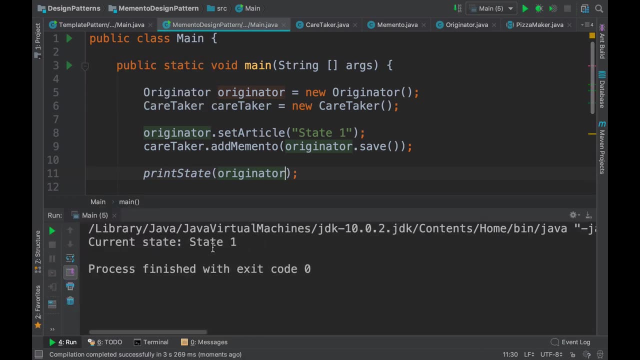 originator. So we are passing this originator and now let's try to run this program and let's see what happens. So, if you see, our program is displaying current state, state 1.. So, since this is the only state, it is actually displaying this. So now let's go ahead and try to add more. 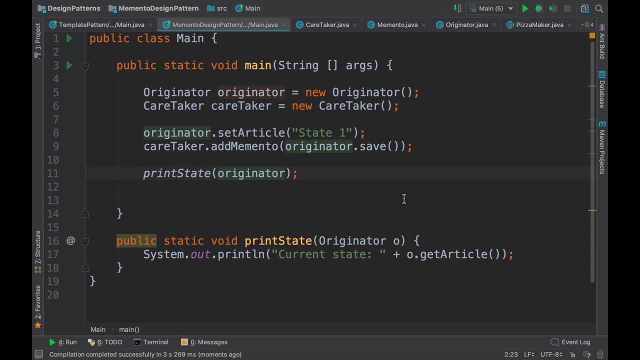 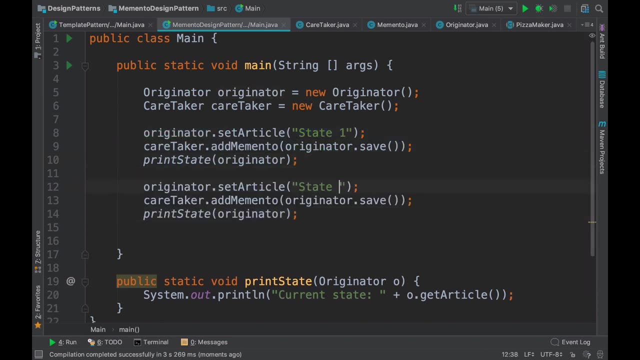 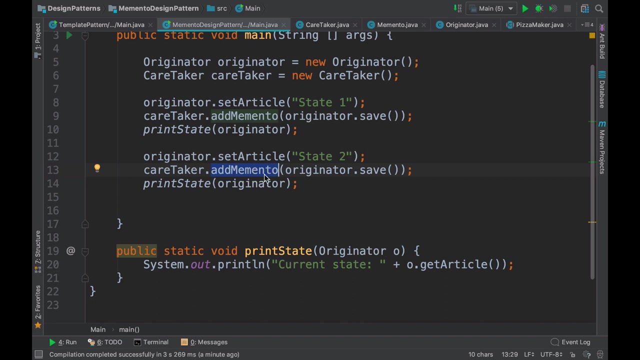 states to this program and then apply undo and redo methods on it. Let me copy this code here and let's add a state 2 and ask the caretaker object to add the memento here. And since this will again implement, current state is state 2, let's go ahead and 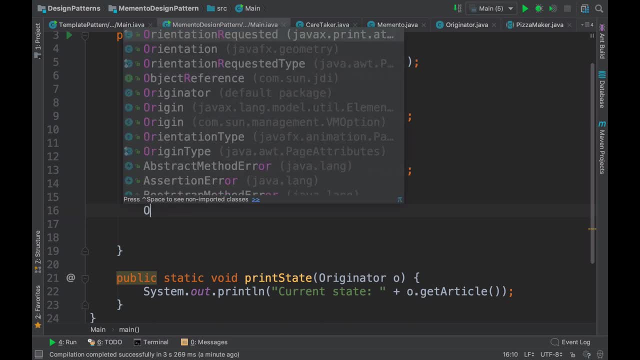 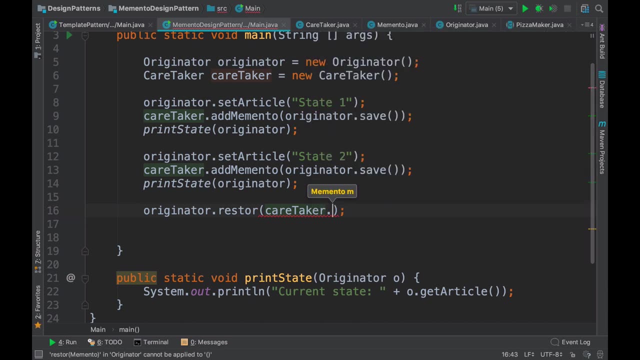 add some undo and redo methods. So what I want to do is originator dot restore. I want to restore this state and what I'll say here is caretaker dot undo. So now, what caretaker dot undo will do is it will point the current cursor of the state to the previous state for whatever it was in the 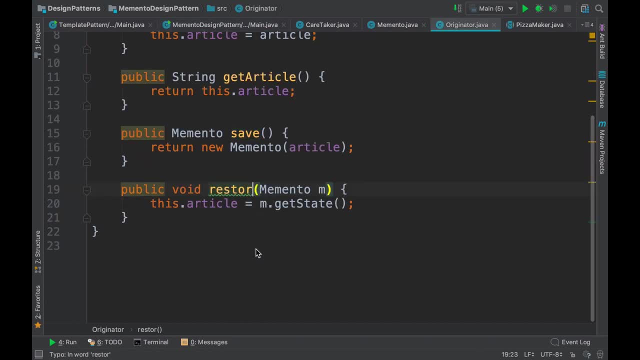 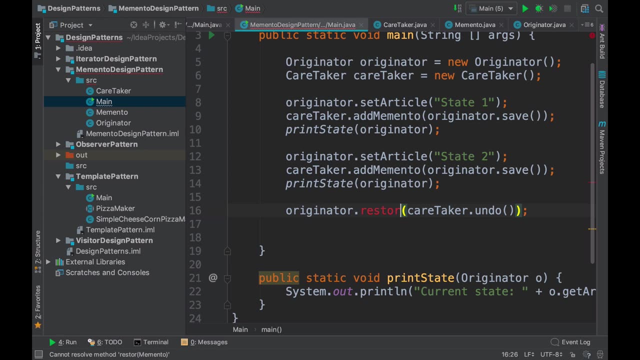 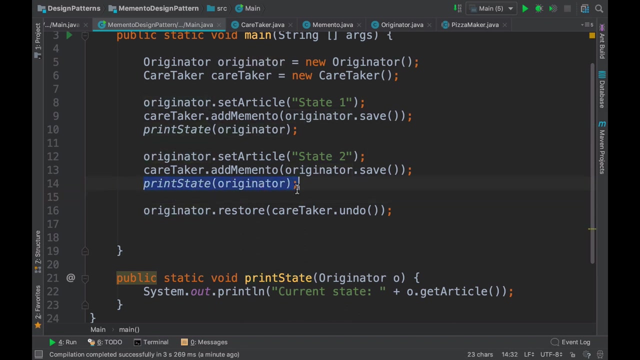 position. So I think I have named this variable incorrectly, So let me go ahead and correct it. And now let's go to the main method and say: restore here. So now, if you go ahead and print the state for the originator, 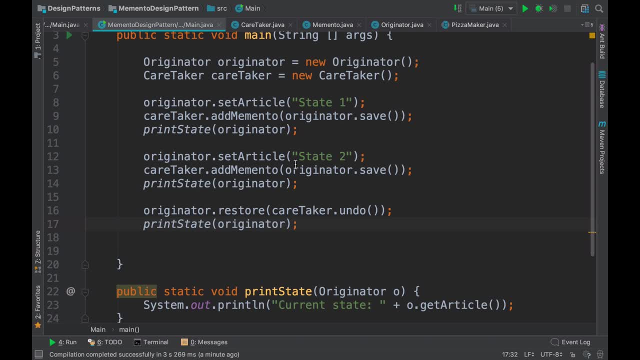 what we will see is: we will see: current state is state 1, because we already set the article to state 1.. It added a new state, Then we modified the state to state 2. And then we are doing an undo, So it will again roll back this change and it will come here. 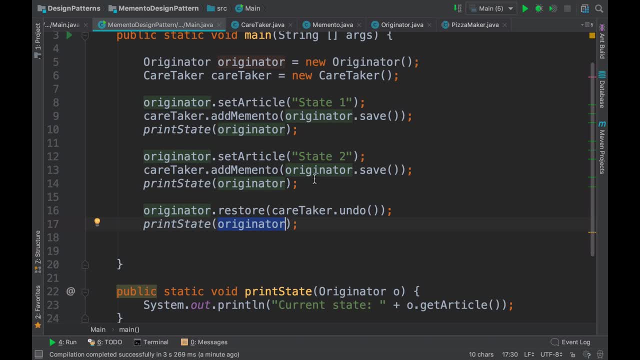 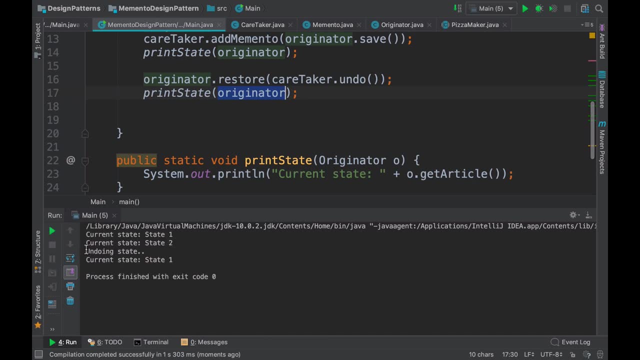 And this: if you try to print the current state of this originator, you will see state 1.. So let's run this program and it should show state 1.. So now you see that we have this small little text to undoing this state And after undoing this state, you see that current state of the originator. 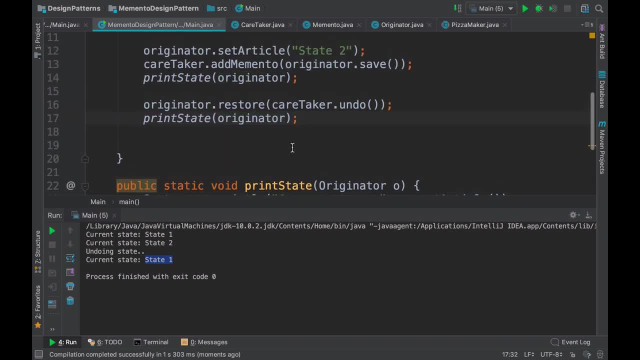 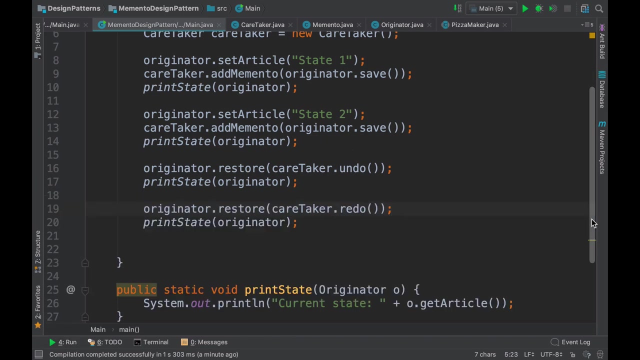 is state 1.. Now you have seen that the undo methods works perfectly. Now, at this point of time, we know that our current state is state 1.. So now, if we try to do a redo here, it will again go forward in time. So it jumped from state 2 to state 1 when we did an undo. 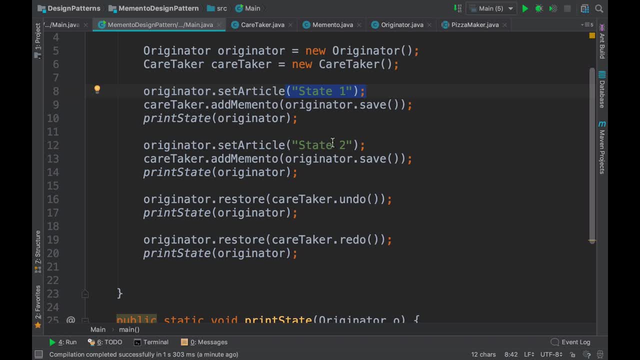 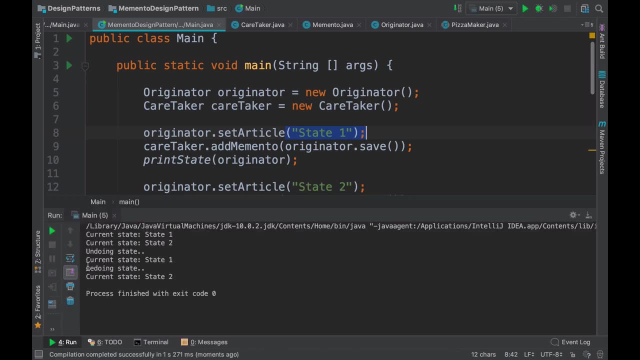 Now, if we do a redo here, it will again jump from state 1 to state 2.. Now let's go ahead and run this program and see this in action. So yeah, so after redoing state, you see that the current state again jumps back to state 2.. So now you can play around with. 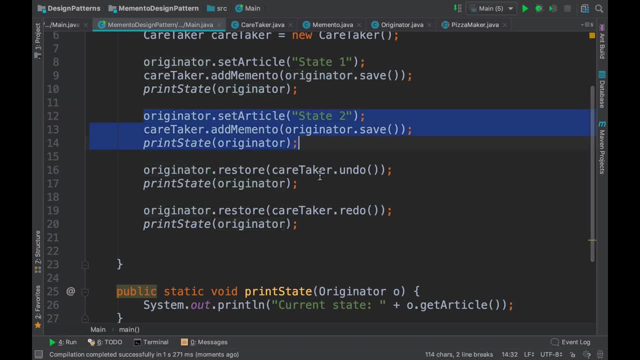 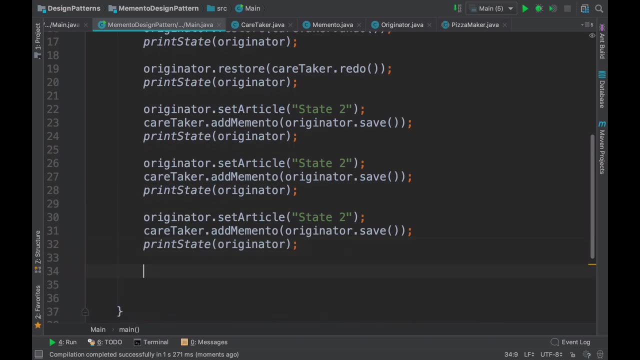 this, creating multiple states, and enjoy going backward and forward. So let me create some four or five states here, and let's call it three, Let's call this four, Let's call this five and let's call this six. Now, at this point of time, our current state is state six, So let's 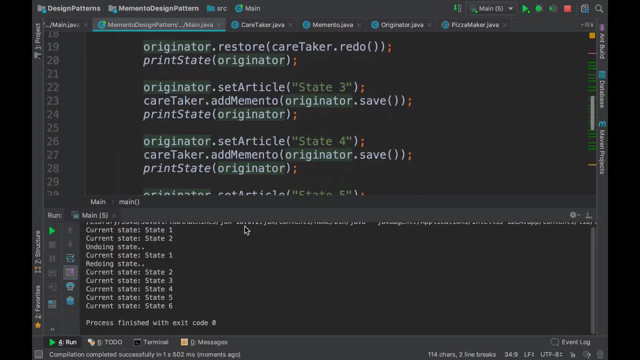 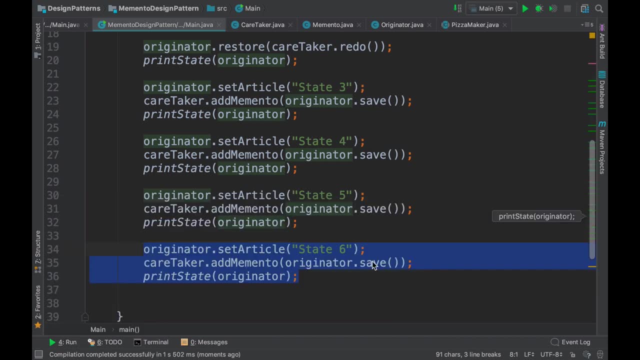 run this program and see this in action, We'll see that current state is state six. Now, from here, if we undo three times, we should go back to current state four. So let's go back and try to do an undo to reach state four. 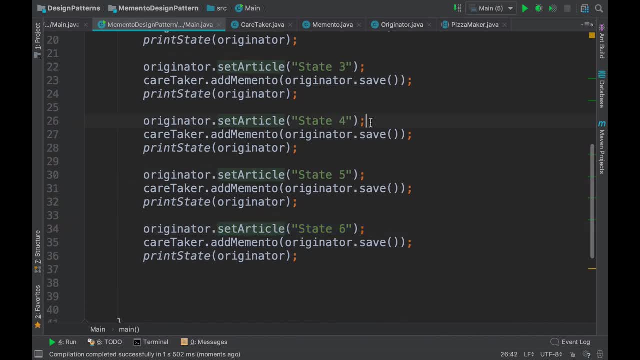 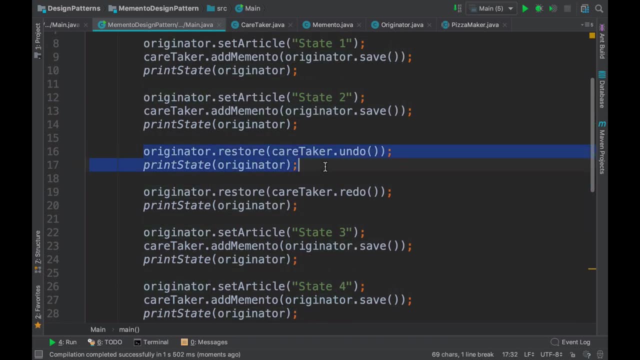 Sorry, if we do undo three times, we will not be having state four, we will be having state three. So now let's go ahead and just do an undo over here, So we'll copy our undo code And instead of printing each undo, let's 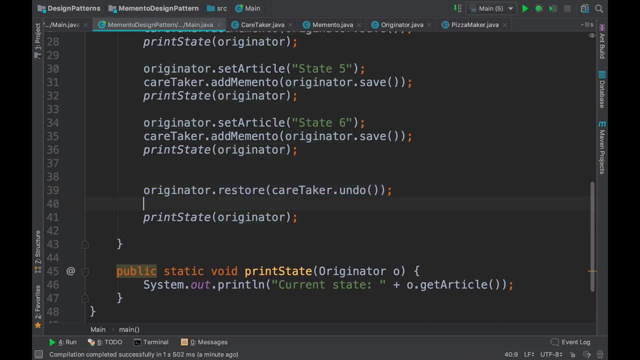 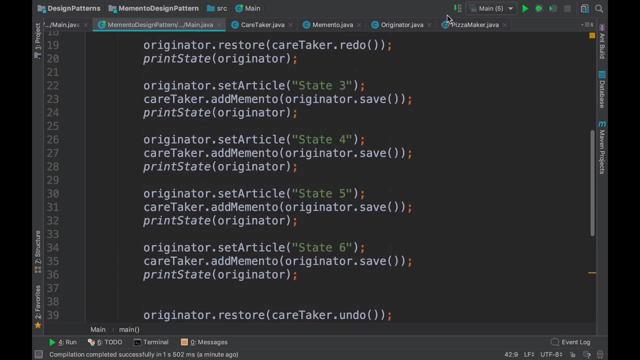 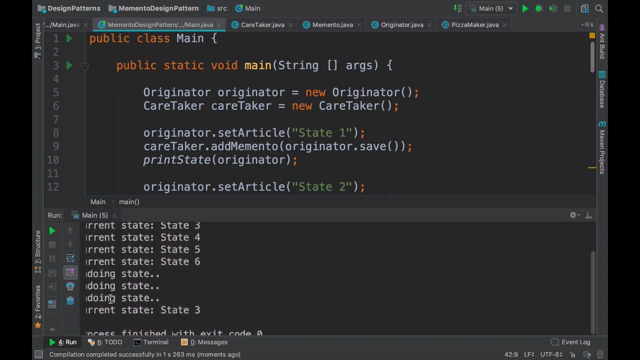 only print after we are done undoing a certain number of times. So here we want to undo our state times, so let's undo three times and then print the state. so now we'll be getting state 3. let's go ahead and run this and, yeah, we are again back to state 3. so 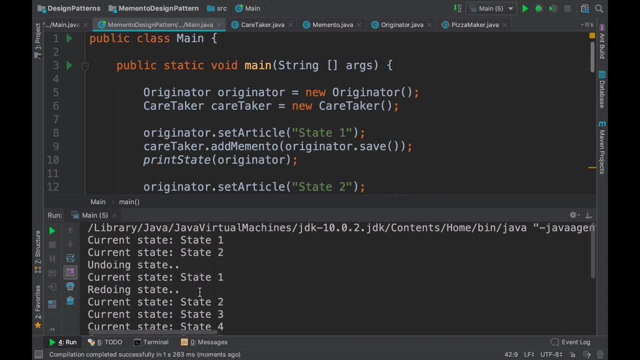 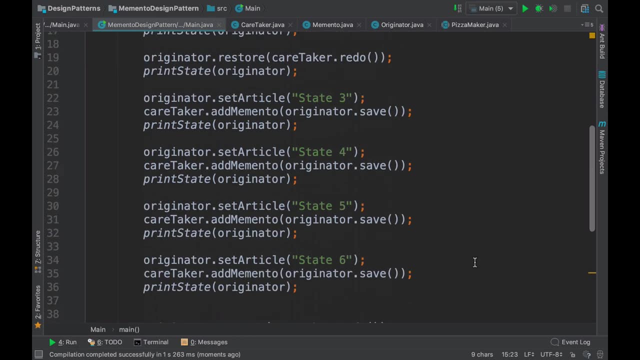 from 1 we went to 2, then we again went back to 1 and 2, 3, 4, 5, 6, then we did undo three times. we are at state 3 now. let's try one more time. let's try redoing this. 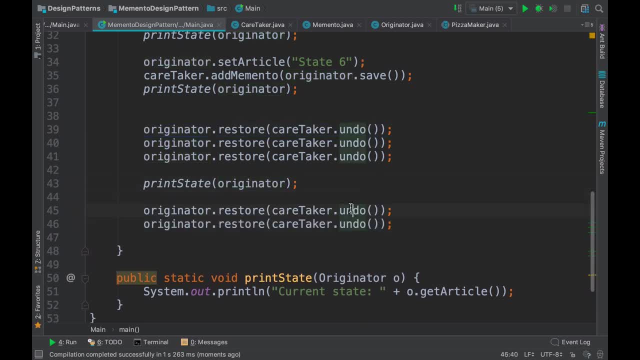 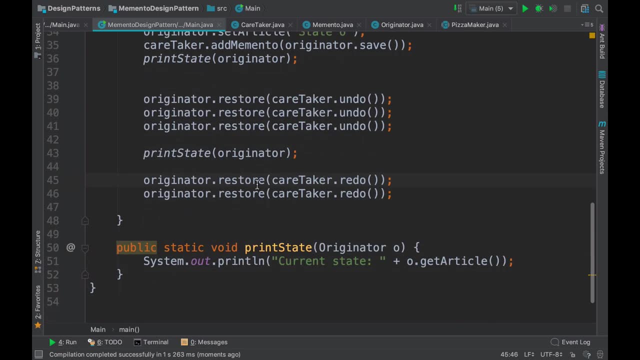 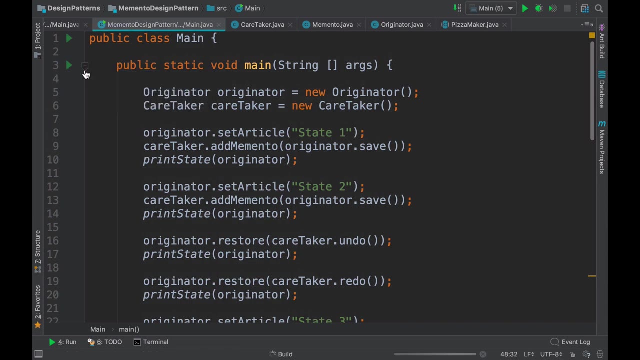 two more times. so if we redo what we undo two more times, we'll be again back to state 5. so to finally see the answer, we need to print the state. so let's go ahead and actually do it. so now you see that after redoing state, we are again. 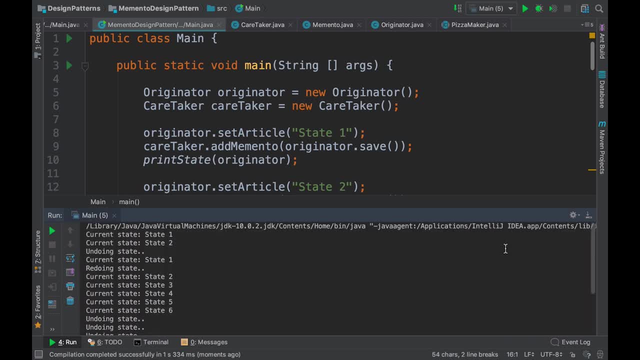 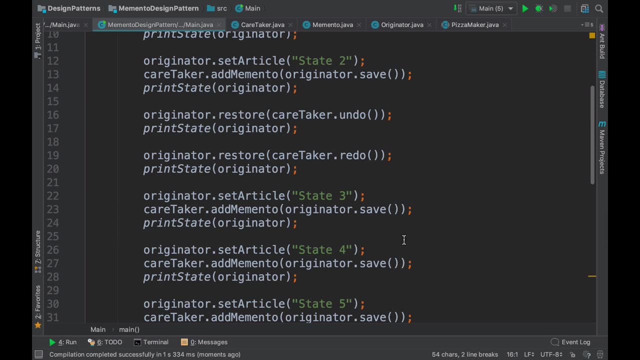 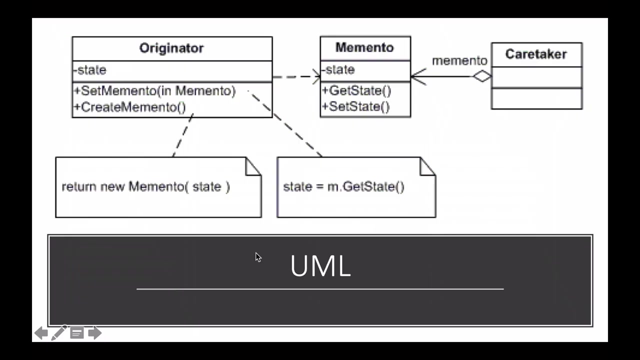 back to state 5. so this is the memento design pattern. it lets you save memories of your object somewhere so that you can restore, go forward in memory, go backward in memory and just do whatever you want with that saved application state. so this is what memento design pattern is trying to solve. it gives you an elegant way to 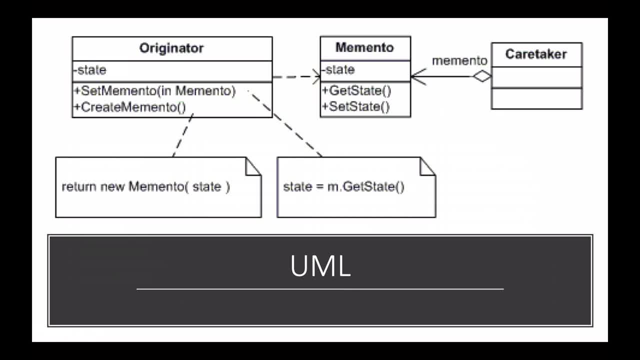 actually go forward and backward depends on your use case. let's say you are designing a text editor application and you want to save the state for this modified text. you can keep your state in the memento and just on ctrl-z or undo operation or on a redo operation you can just go through the set of operations. 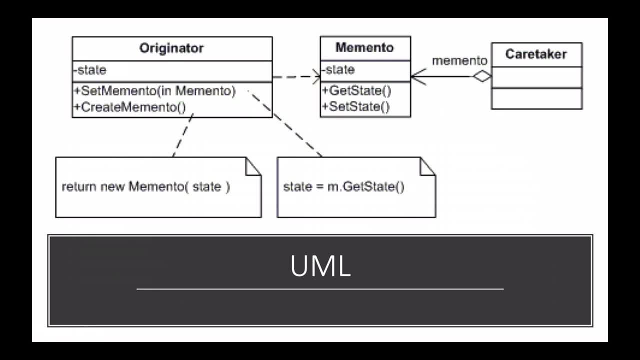 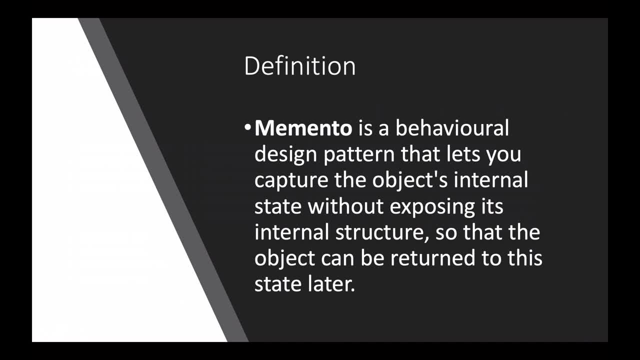 you already go through the set of states you already have persistent in your caretaker. so I hope you have understood what this memento design pattern is. its a behavioral design pattern, as you all know, and it lets you capture the objects internal state without exposing its internal structure. 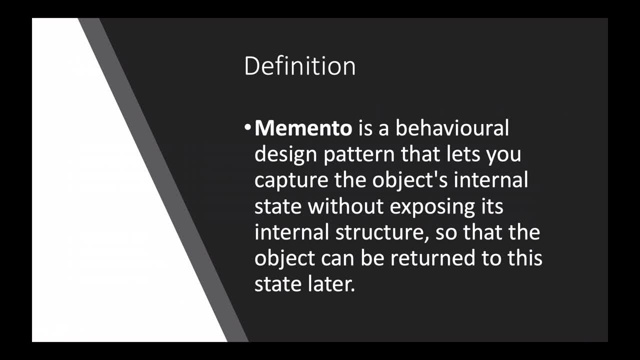 so that the object can be returned to this state later. and here you are with the memento design pattern, with implemented from scratch using all these four steps. so that's it with the memento design pattern. I hope to see you in the next one.